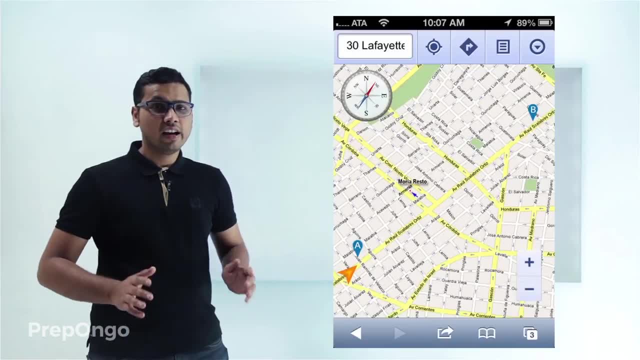 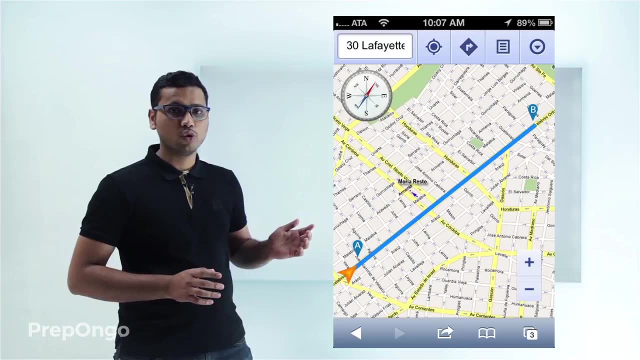 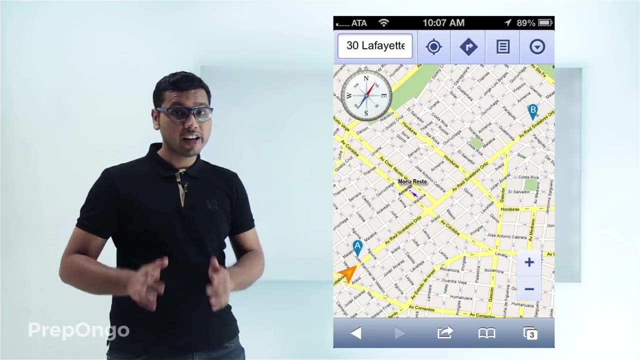 Hello everyone. let's suppose that you are going from city A to city B and you are looking at your GPS to know the distance between A and B. So after some time, all of a sudden, your GPS malfunctions and you are unable to find the distance between A and B. but you 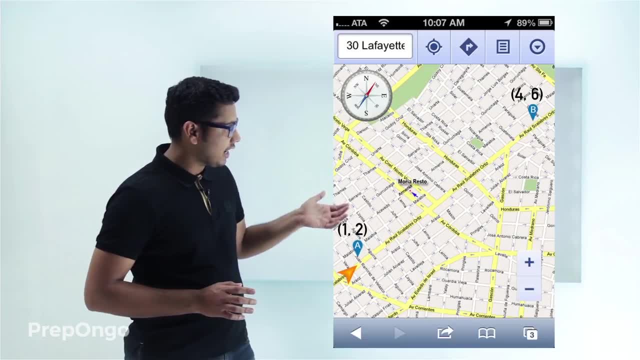 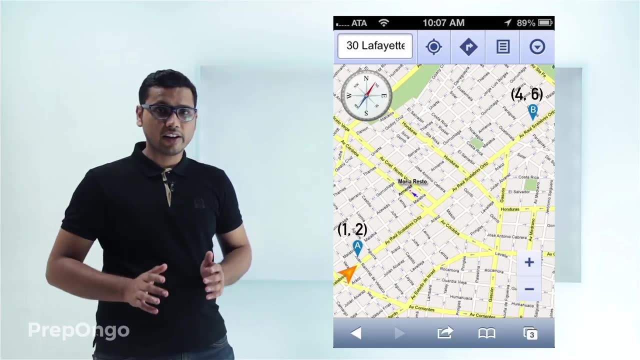 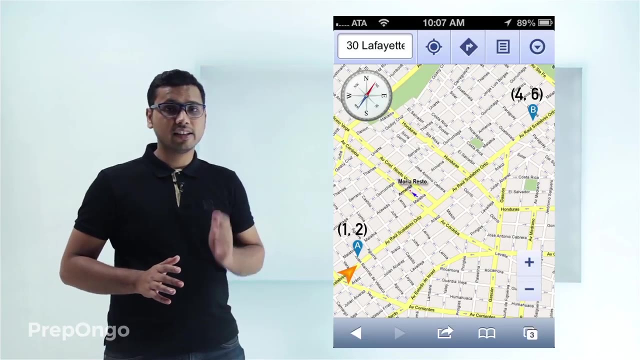 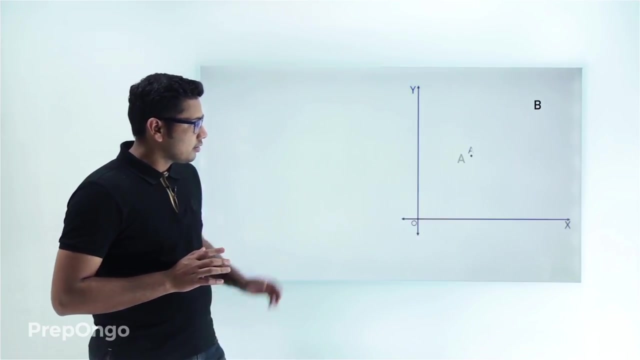 are able to find the coordinates of city A and city B. So how will you calculate the distance between these two cities? So let's have a method which establishes a relation between the coordinates of two points and the distance between these two points. So let's bring out our coordinate axis and let's say that point A and point B represent 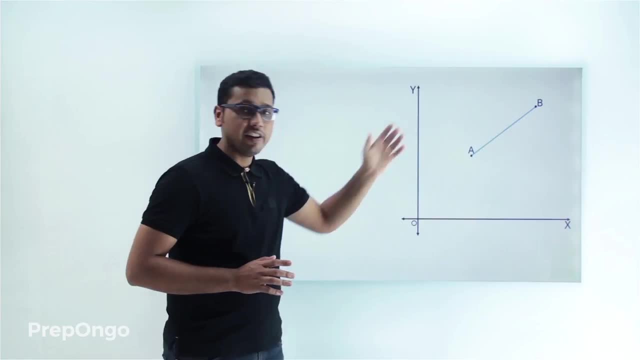 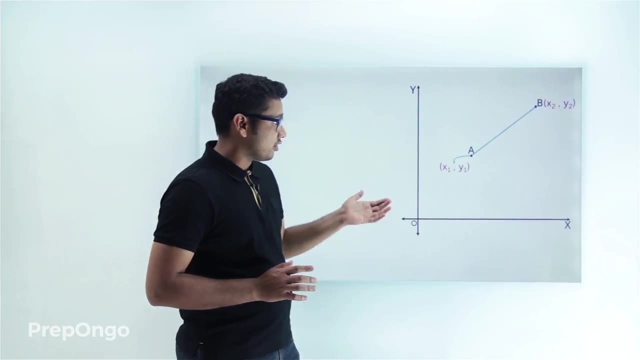 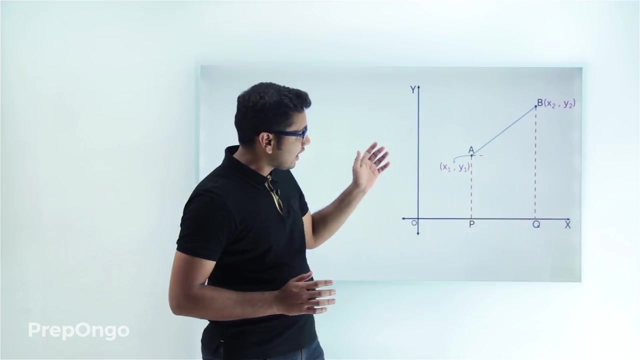 the cities. So this distance AB we have to calculate if we know the coordinates of point A and point B coordinates is x1 comma y1 and b coordinates are x2 comma y2.. Now let's have some constructions to find the length AB. So I had drawn AP and BQ perpendicular to x-axis and AR perpendicular to. 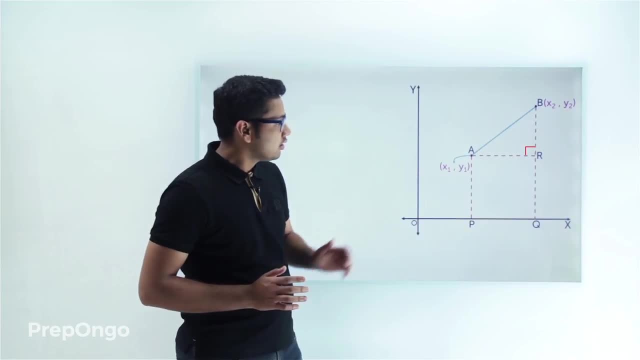 BQ line. So we can find out the length of AB in triangle ARB. Now this triangle is a right angle triangle, So we can always apply Pythagoras theorem in this triangle. So Pythagoras theorem says that hypotenuse square is equals to the sum of square of other two sides. So we can say that. 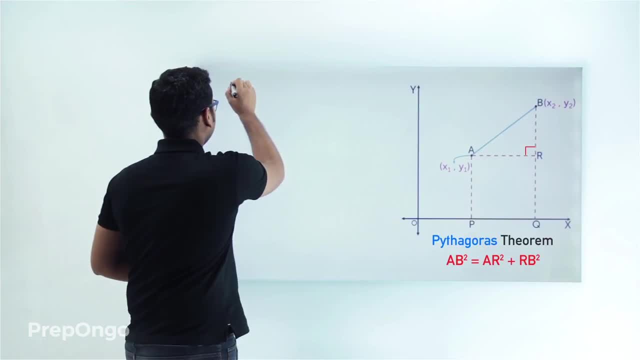 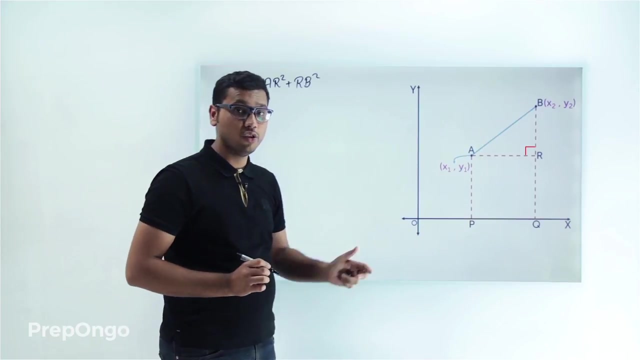 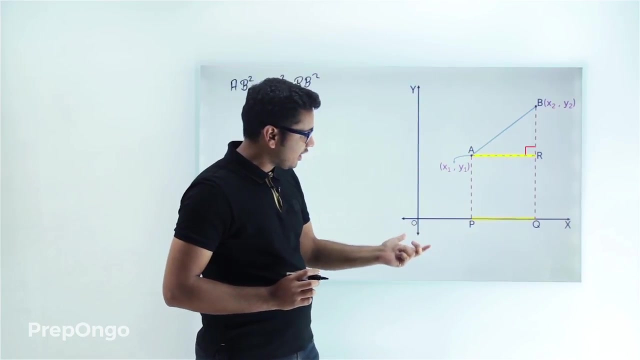 AB square will be equals to. this is equals to AR square plus RB square. And now we can find the values of AR And RB since we know the coordinates of point A and point B. So AR will be equals to PQ and we can find the length PQ as OQ. we know this is x2 and OP is x1.. So the length AR will become to be x2. 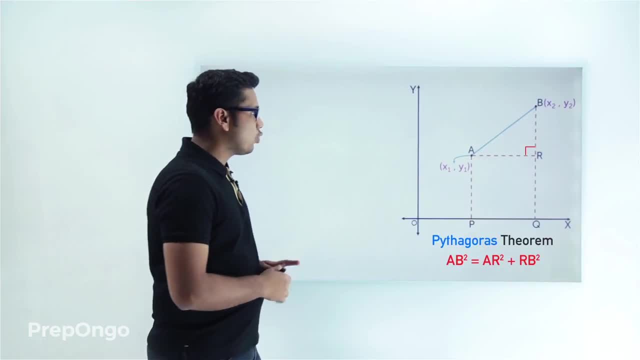 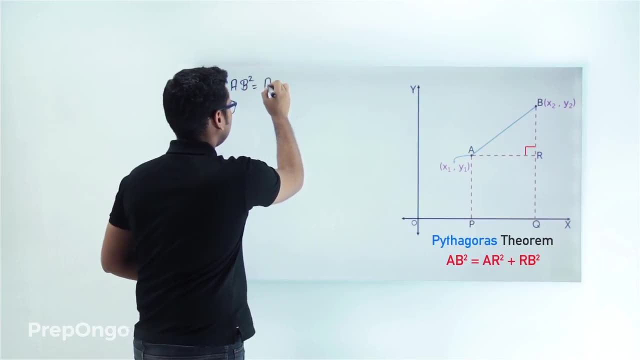 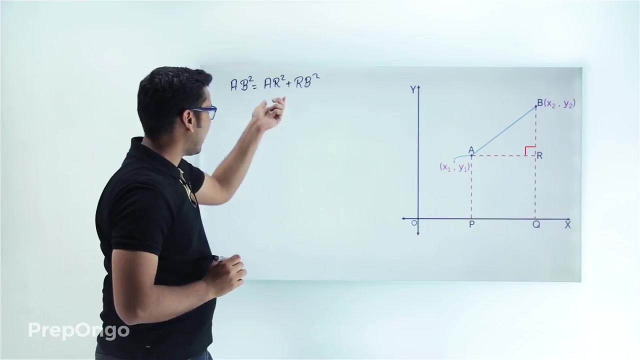 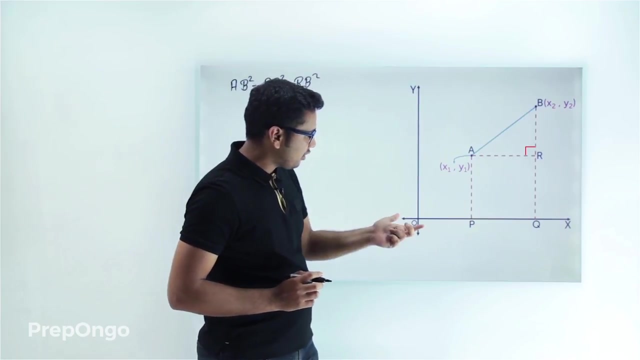 two sides. So we can say that AB square will be equals to. this is equals to AR square plus RB square. And now we can find the values of AR and RB, Since we know the coordinates of point A and point B. So AR will be equals to PQ and we can find the length PQ as OQ. we know this is x2 and 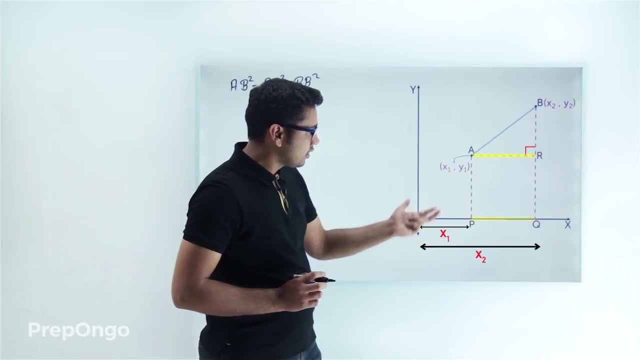 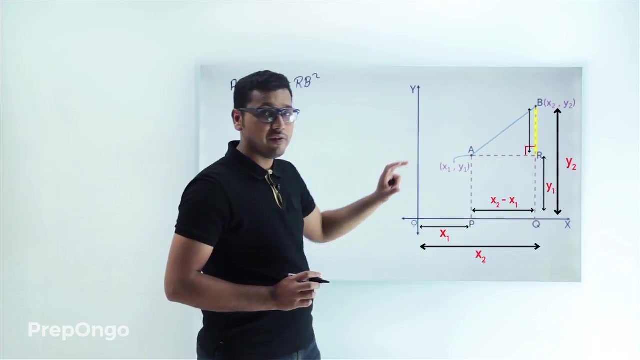 OP is x1.. So the length AR will become to be x2 minus x1.. Similarly we can find the length RB. We know BQ is y2 and RQ is y1.. So this length RB is y2.. RB will become y2 minus y1.. 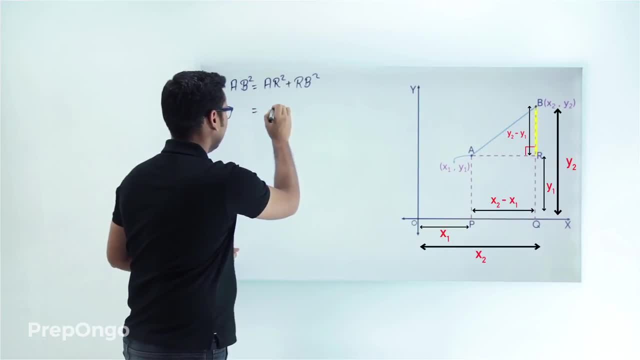 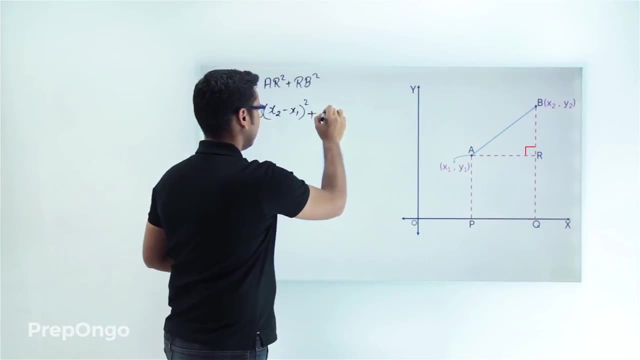 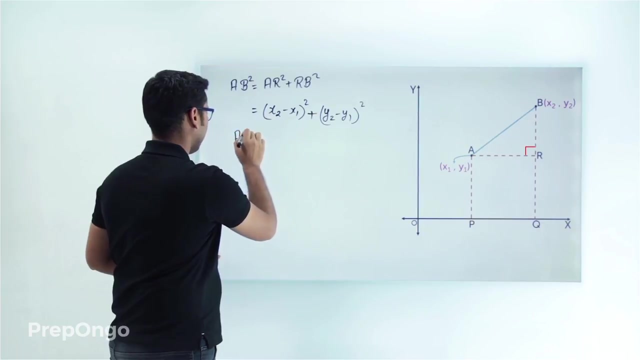 So let's put the values, This will be x2 minus x1 whole square plus y2 minus y1 whole square. Now if we have to find out the length AB, So let's take the under root on both the sides. So this will become x2 minus x1 whole square plus y2 minus y1 whole square plus y2 minus. 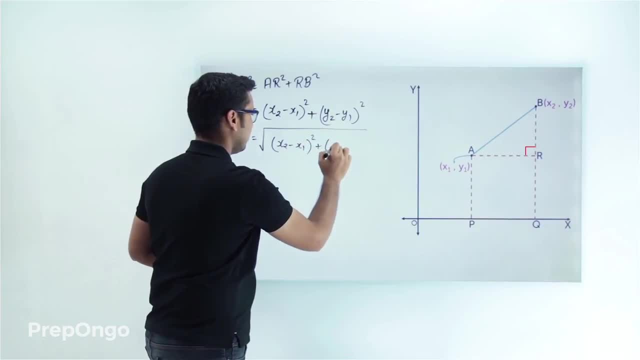 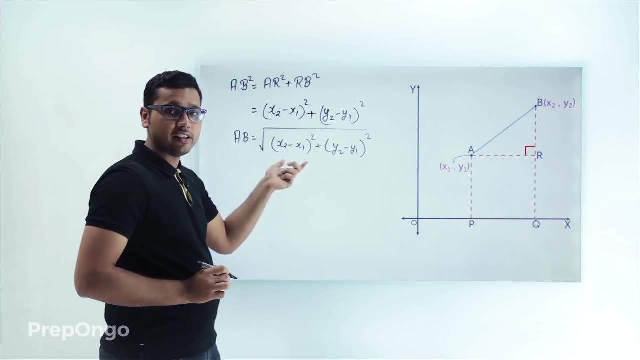 y1 whole square. Now if we have to find out the length AB, So this will be x2 minus x2 plus y2 minus y1 whole square plus y2 minus y1 whole square. Now if you see that if we take the negative sign common from this term, it will square. 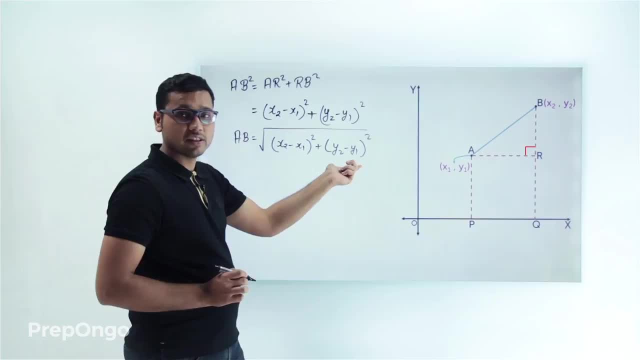 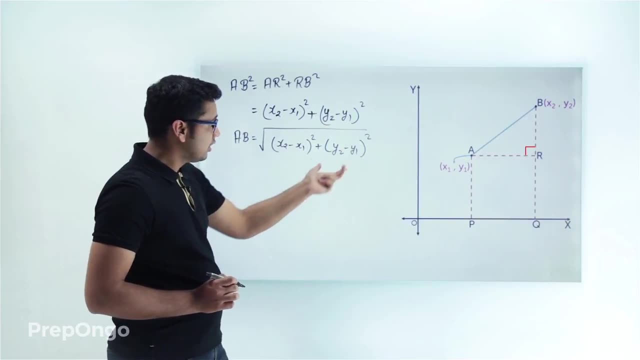 and become positive. Similarly, from this term, this will also become square and become positive. So instead of this, we can also write x1 minus x2, and instead of this, we can also write y1 minus y2.. So this is equivalent to. So this is equivalent to. 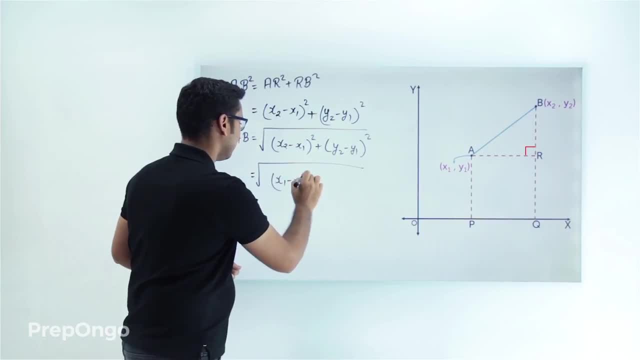 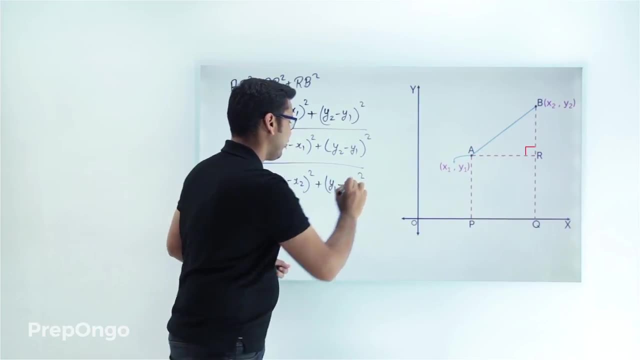 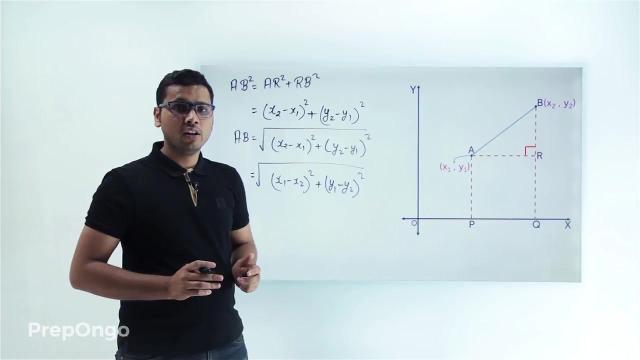 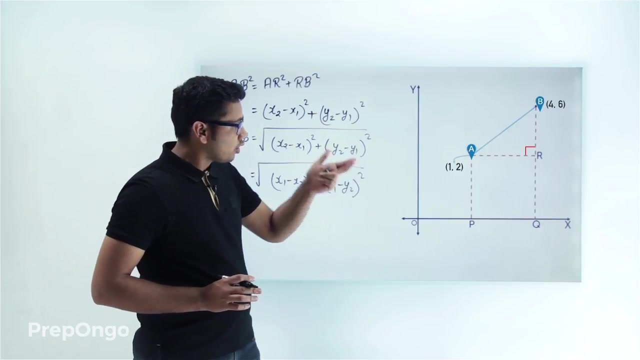 So this is equivalent to x1 minus x2 whole square plus y1 minus y2 whole square, and we can apply either result to find the distance between any two points if their coordinates are given. So let's find out the distance between city A and city B. We knew that the GPS was showing coordinates of city A to be. 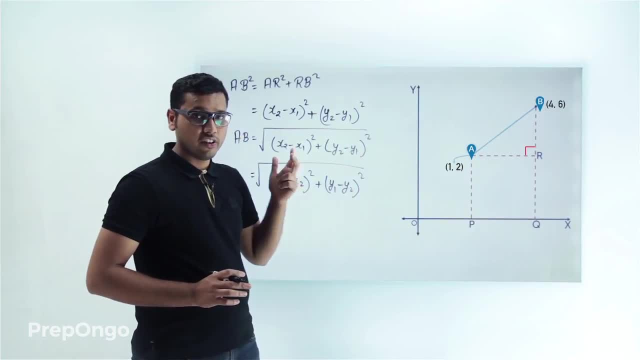 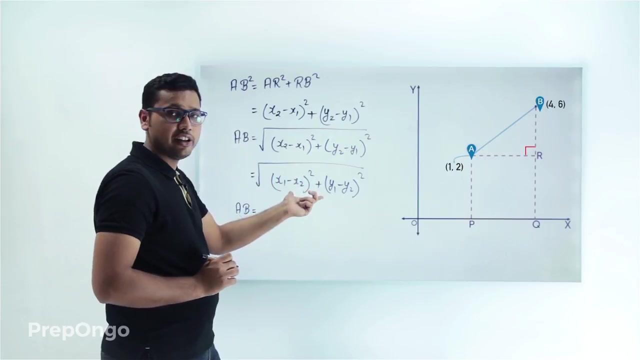 1 comma 2 and coordinates of city B were 4 comma 6.. So let's apply these values and find out the distance A B, So A B will be equals to. let's apply the second relation to find out the. 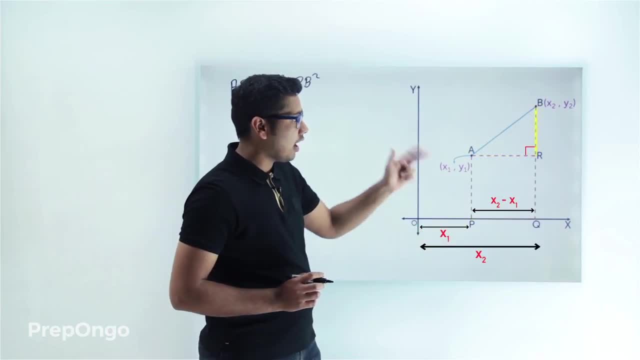 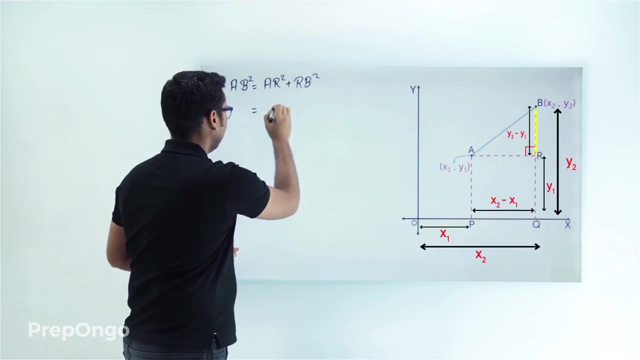 minus x1.. Similarly we can find the length RB. We know BQ is y2 and RQ is y1.. So this length RB will become y2 minus y1.. So let's put the values, This will be x2 minus x1, whole square plus. 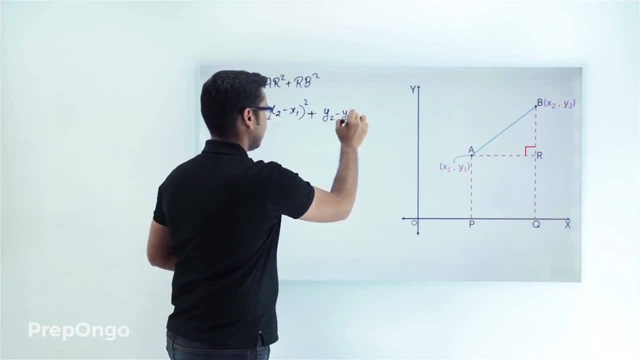 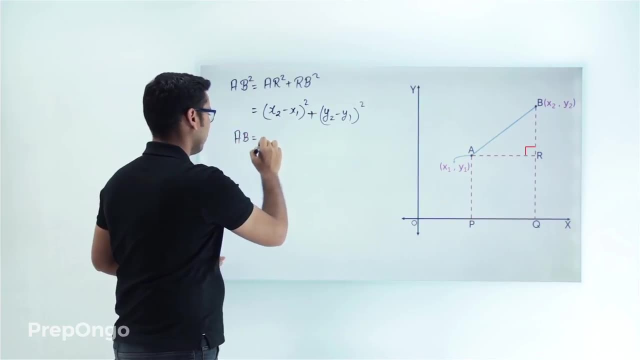 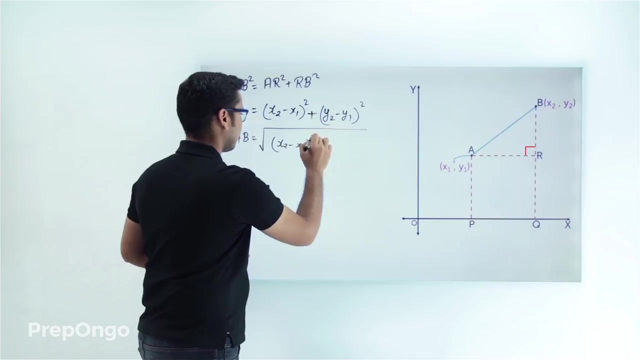 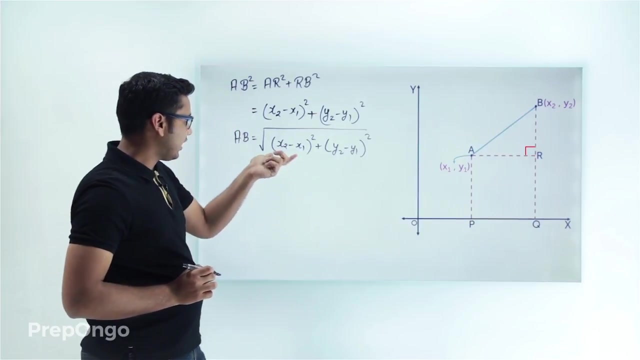 y2 minus y1- whole square. Now if we have to find out the length AB, So let's take the under root on both the sides, So this will become x2 minus x1- whole square square, plus y2 minus y1- whole square. Now if you see that, if we take the 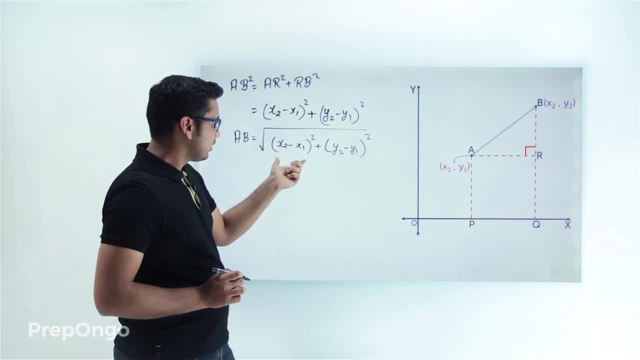 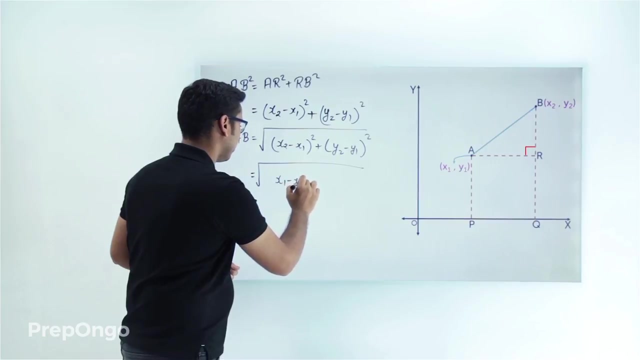 negative sign common. from this term, it will square and become positive. Similarly, from this term, this will also become square and become positive. So instead of this we can also write x1 minus x2, and instead of this we can also write y1 minus y2.. So this is equivalent to x1 minus x2, whole square plus y1. 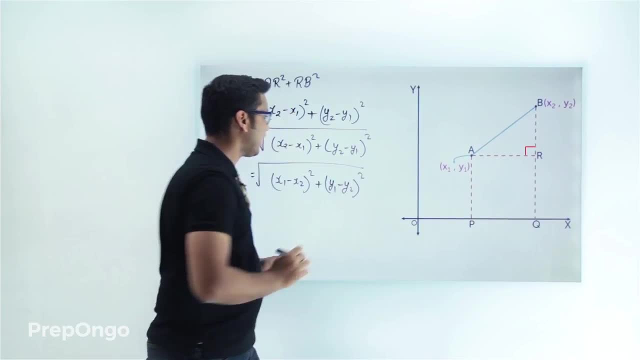 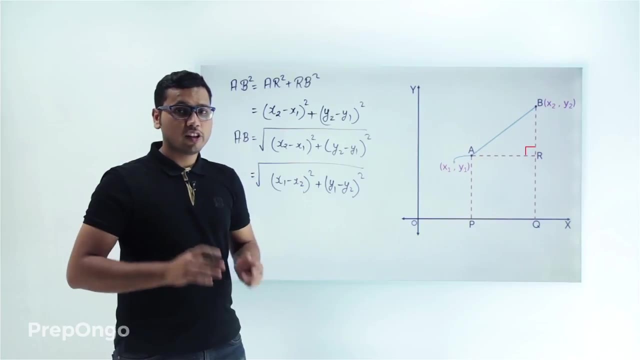 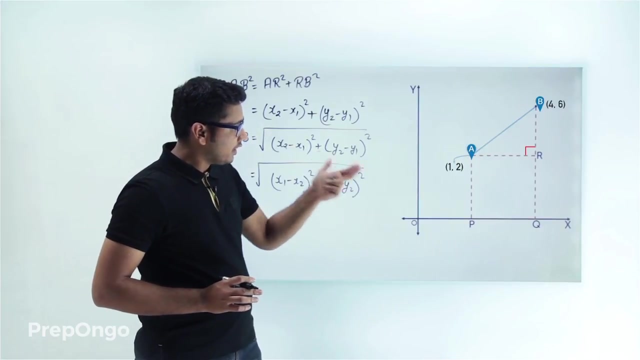 minus y2, whole square And we can apply either result to find the distance between any two points if their coordinates are given. So let's find out the distance between city A and city B. We knew that the GPS was showing coordinates, Coordinates of city A to be 1 comma 2 and coordinates of city B were 4 comma 6.. 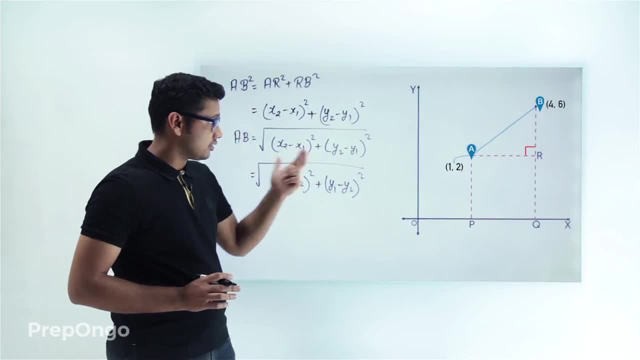 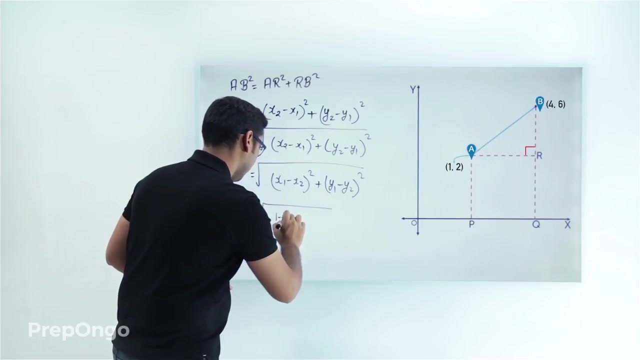 So let's apply these values and find out the distance ab. So ab will be equals to. let's apply the second relation to find out the coordinates, So this will be under root: 1 minus 4, x1 minus x2, so x1 is 1. 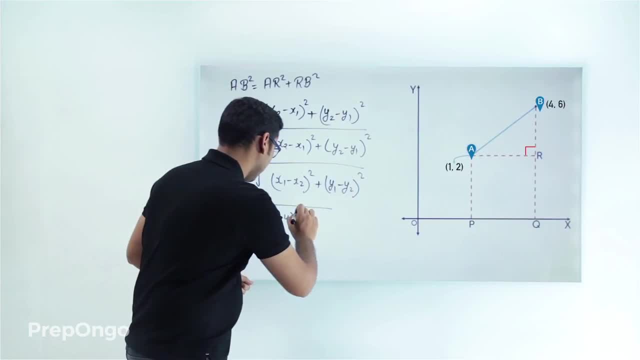 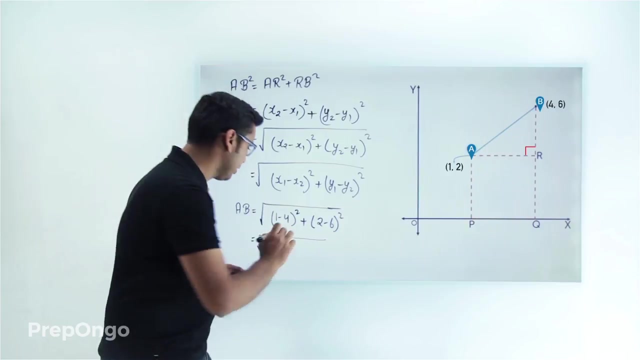 X2 is 4.. 1 minus 4: whole square, plus y1 minus y2: whole square: x1 is 2 and y2 is 6.. So now let's solve this. This is 1 minus 4, so this will become minus 3, and minus 3 square is 9, so this will be 9, and just find the.